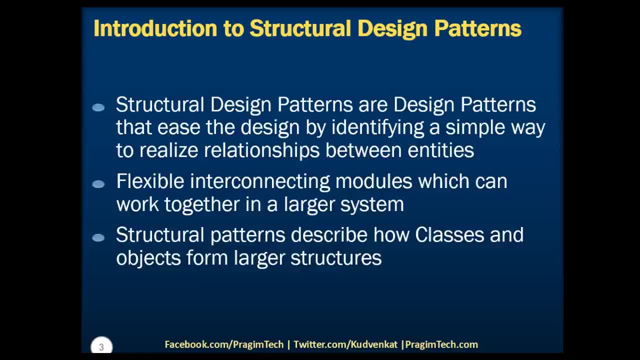 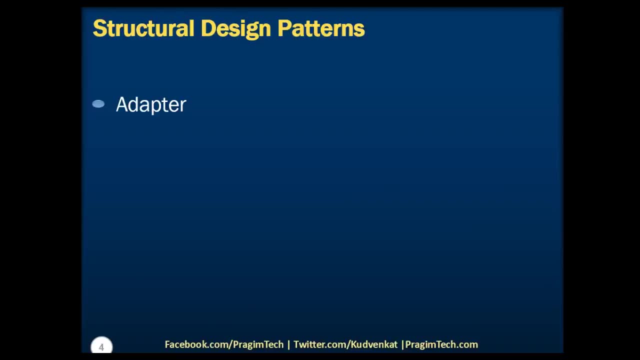 describe how objects can be composed into larger structures using object composition or the inclusion of objects within other objects. Ganga 4 has identified seven structural design patterns, which are: adapter, bridge, composite, decorator, facade, flyweight and proxy patterns. Let's now look into the definition of these patterns. 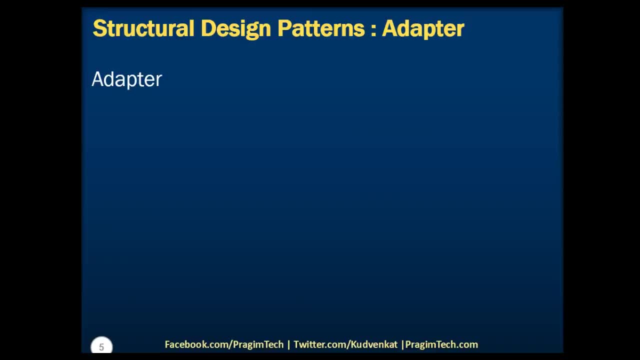 As per the ganga 4 definition, adapter match interface of different classes. To simplify this definition, we can state that an adapter allows two incompatible interfaces to work together, which means the adapter design pattern allows incompatible classes to interact with each other by converting the interface of one class into an interface. 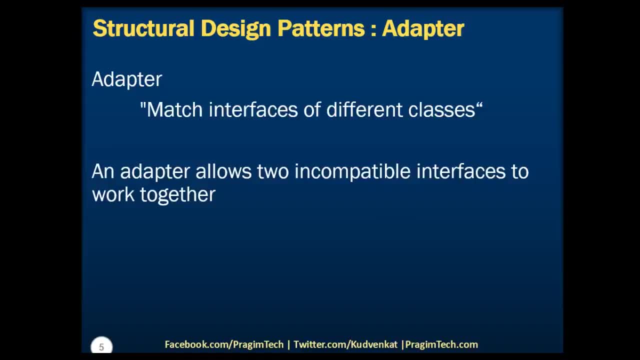 which is expected by the end clients. leveraging on adapter improves reusability of older functionality. we will discuss this in detail in next coming sessions. let's now focus on bridge pattern. as per gang of four definition, bridge pattern separates an object's interface from its implementation. to simplify this definition, 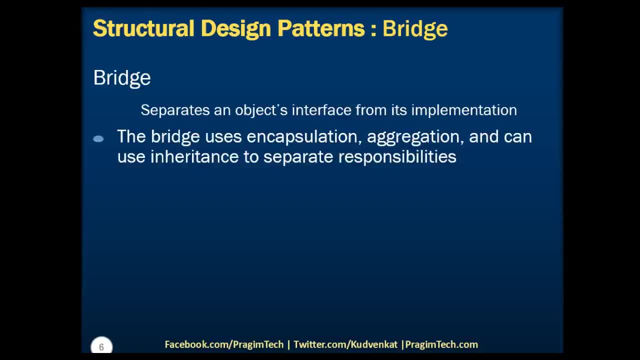 the bridge pattern uses encapsulation- aggregation, and can use inheritance to separate responsibilities into different classes. bridge pattern decouples an abstraction from its implementation so that decoupling and abstraction can vary independently. the bridge pattern can also be thought of as two layers of abstraction. the bridge pattern is useful when we want to avoid 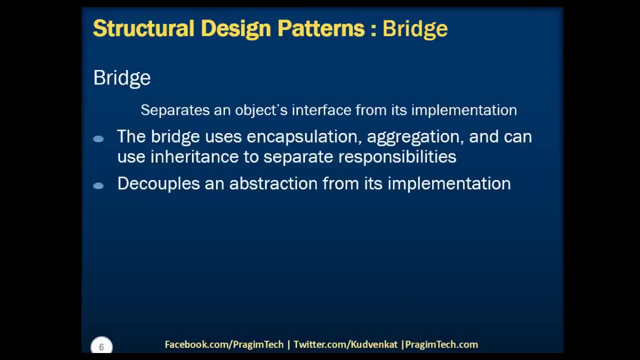 a permanent defended decappulation to ensure believability of a fruits of the subject's abstraction. binding between an abstraction and its implementation Bridge pattern enables us to separate the interface from the implementation and improves extensibility. Also, it hides implementation details from clients. Let's now look into the composite pattern. 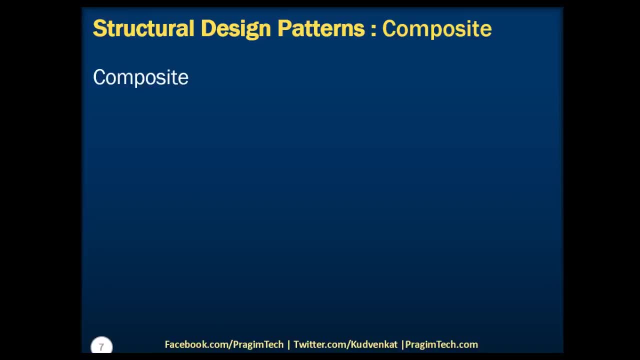 As per Ganga 4 definition, composite design pattern constitutes a tree structure of simple and composite objects. In object-oriented programming, a composite is an object designed as a composition of one or more similar objects all exhibiting similar functionality. The composite pattern enables us to create hierarchical tree structures of varying complexity while allowing 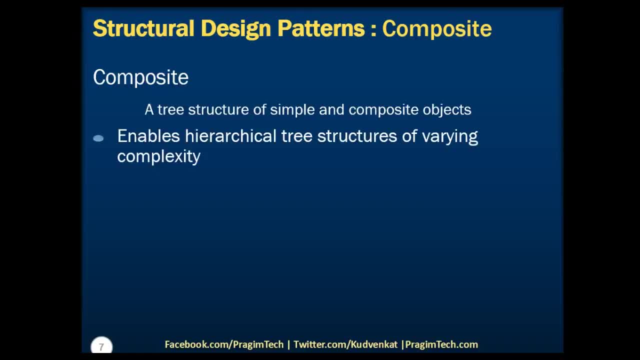 every element in the structure to operate with a uniform interface. The composite design pattern describes that a group of objects are to be treated in the same way as a single instance of an object. The intent of a composite is to compose objects into tree structures to represent part-whole hierarchies. Implementing 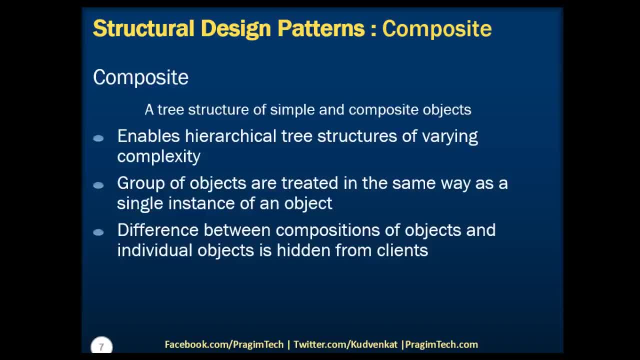 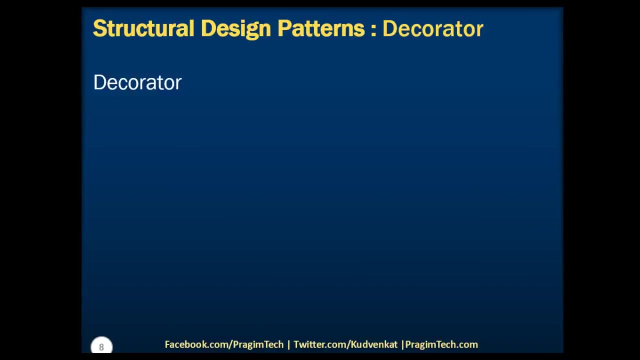 the composite pattern lets clients treat individual objects and compositions uniformly. If this is confusing at this point of time, don't worry. we will take a look at this into greater details, with simple examples, in the coming lectures. Let's now switch to decorator pattern. As per Ganga 4 definition, the decorator pattern. 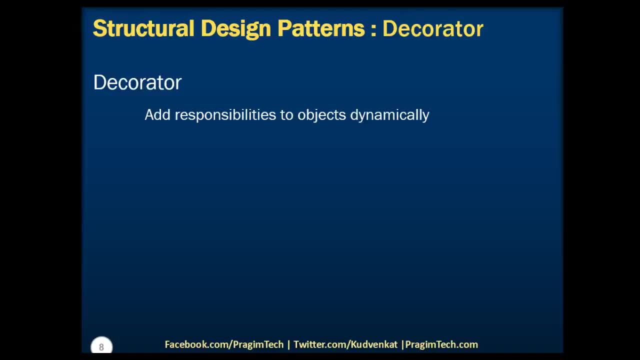 adds responsibilities to objects dynamically. To simplify this, we can state that the decorator pattern enables us to add or remove object functionality without changing the external appearance or function of the object, Which means the decorator pattern attaches additional responsibilities to an object dynamically to provide a flexible alternative. 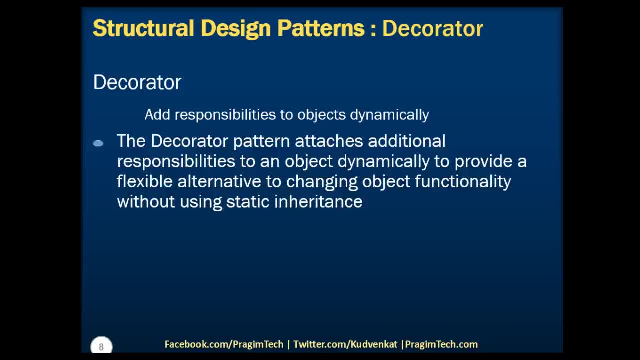 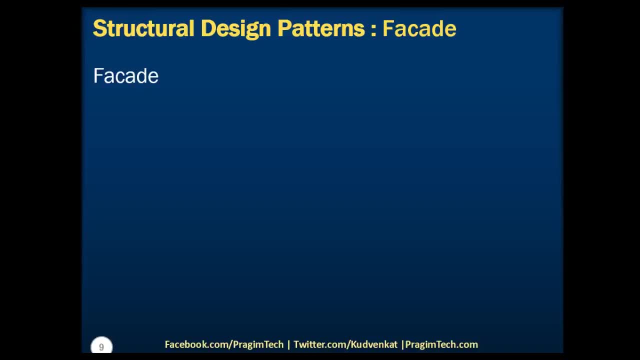 to changing object functionality without using static inheritance. Let's now switch to facade pattern. As per Ganga 4 definition, in the facade design pattern we have a single class that represents an entire subsystem, Which means the facade pattern provides a unified interface to group of interface components in the entities, The. 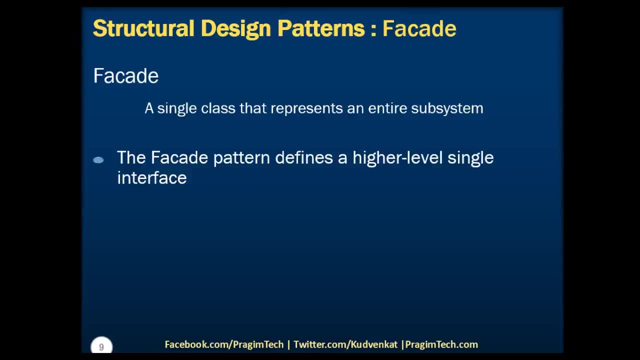 facade pattern uses a single class in order to have a single class in the entire subsystem. The facade pattern provides an interface to a group of interface components and the single interfaces in a subsystem. The facade pattern defines a high-level interface that makes the subsystem easier to use with. 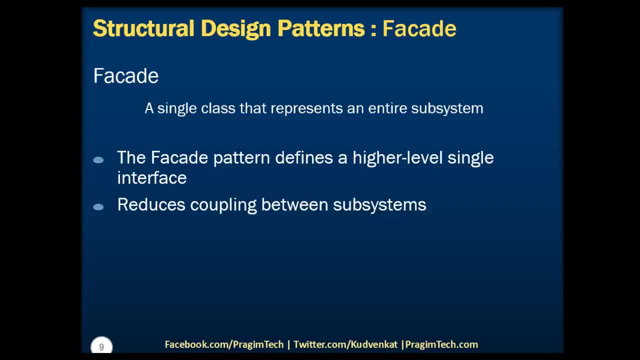 only one single interface. This unified interface enables an object to access the subsystem using the interface to communicate with the subsystem. Facade design pattern reduces coupling between subsystem, provided if every subsystem uses its own facade pattern, and other parts of the system use the facade pattern to communicate.